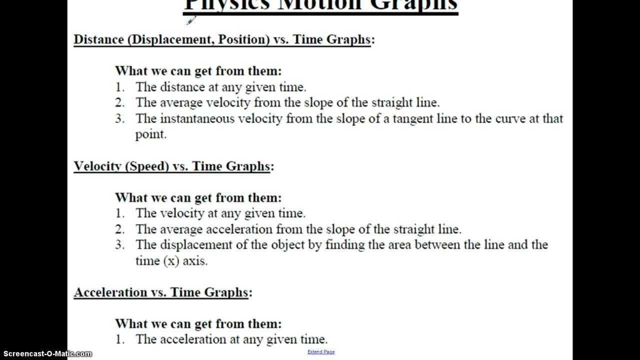 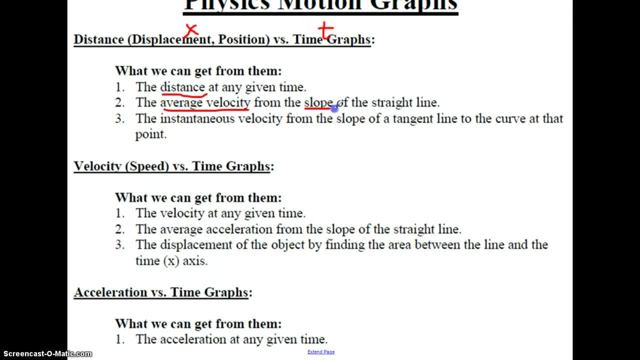 We can also get the average velocity from the slope of the straight line. These two keywords go together: average velocity from slope on a distance time graph, And we can also get the instantaneous velocity from the slope of the tangent line to the curve at that point. So if our best fit line is not a straight line and it's a curve instead, you can see how we can't get average velocity from that, because the velocity is changing. 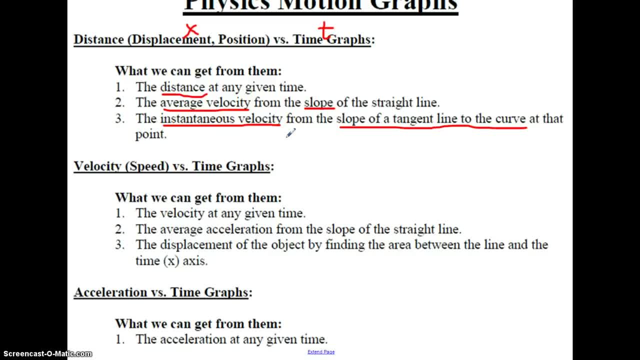 But we would be able to use a tangent line and get the instantaneous velocity using a slope with a tangent, And I'll demonstrate that for you later. Our next type of graph is the velocity or speed, And the same symbol we use for that is V versus time graphs- again T. 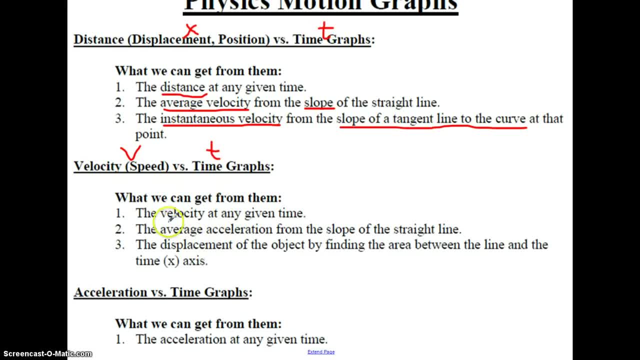 So a VT graph, And what can we get from those? The easiest, of course, again, velocity time graph is the velocity at any given time. Similarly, we get average acceleration from the slope of the straight line, And one thing that is commonly tested is finding displacement of the object by finding the area between the line and the time axis. 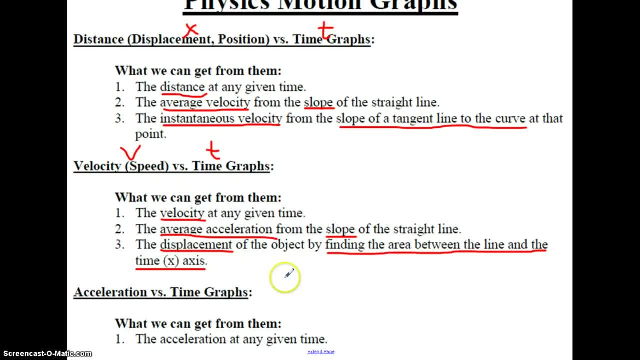 They really like to test that one. Our last type of graph is the acceleration versus time graph. our symbol for acceleration It's A and, of course, versus T, so these would be AT graphs. And what can we get from them? Only the acceleration at any given time. 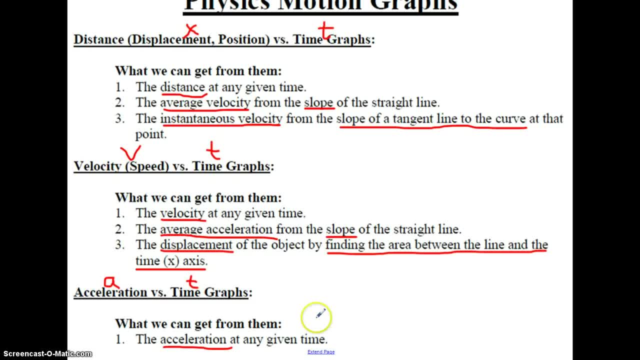 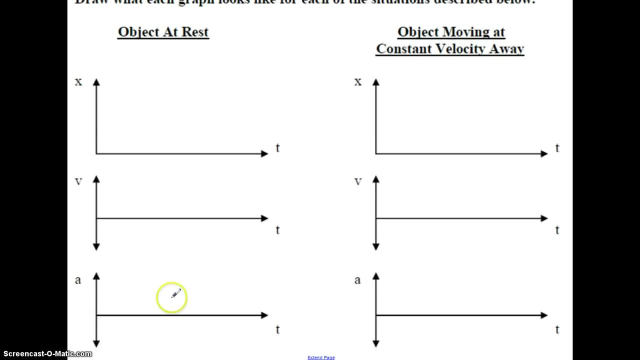 They're the most limited type of motion graph that we can get, as far as the information we can attain from them, And again, I'll demonstrate this for you as we start to do the various graphs for all the types of motion. Let's move on to that and let's take a look at what we're going to do. 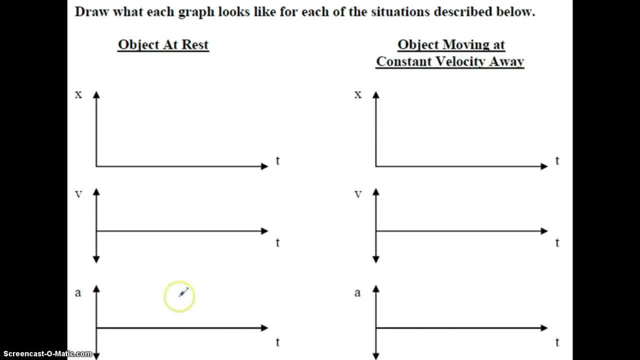 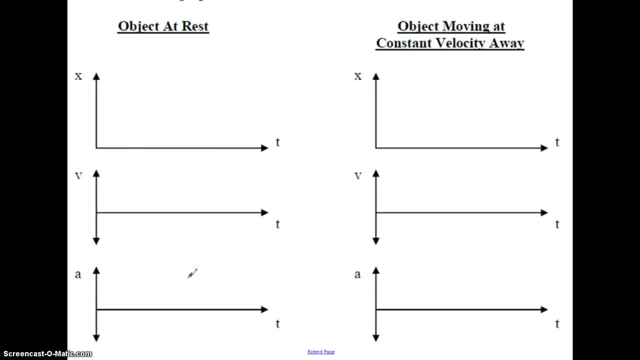 For each of these motion scenarios or situations, we're going to draw the XT, VT and AT graph, one right under the other, so that we have a good understanding of the differences between the graphs and what they communicate to us. So we're going to start with an object at rest. 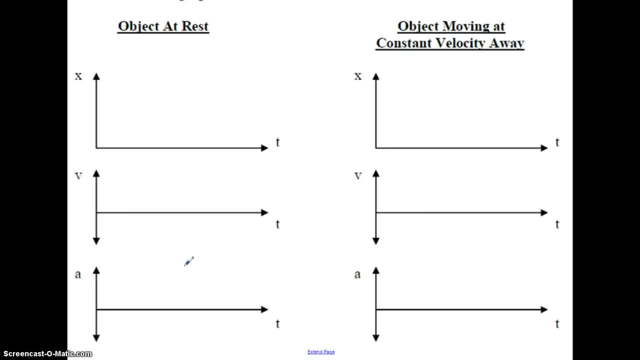 We're going to start easy and work our way towards the harder scenarios. So for an object at rest: if an object is just standing there, that means that its position wouldn't be changing And as time goes forward, so you could pick any spot. 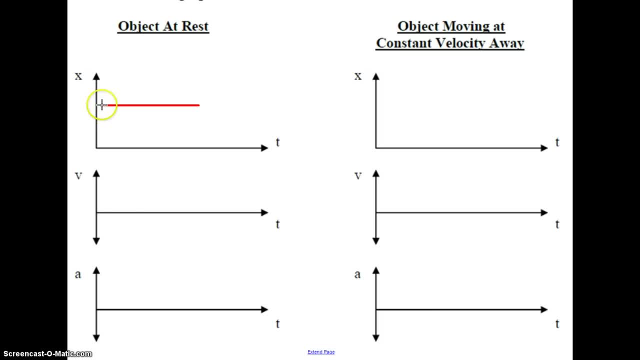 And what this of course means is that the distance is not getting bigger or smaller as time progresses. Well, if an object is at rest, that means its velocity is zero, And where the time axis intersects here on the Y-axis would be where velocity is zero. so we would have a VT graph that has a horizontal straight line on the time axis. 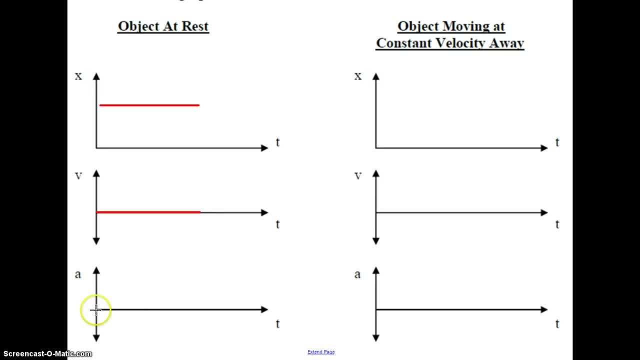 If there's no velocity, there's no acceleration. so it also has a zero AT graph, a horizontal line on the time axis. Okay, We now go to an object at rest. So we're going to start with an object moving at constant velocity away. 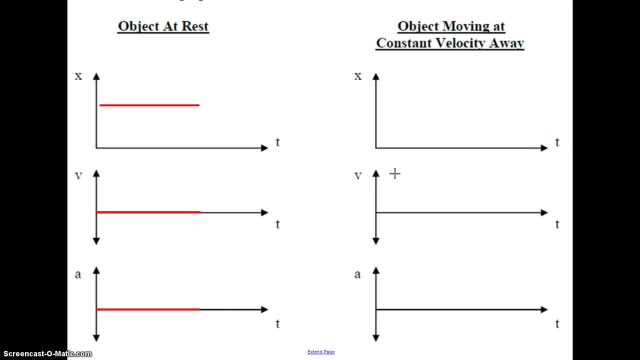 What does that mean? That means the velocity is constant, but the distance is increasing over time. So this, of course, would be a straight line sloped upward. And this: if you take a look, the X numbers are getting bigger, while time is moving in a positive direction. 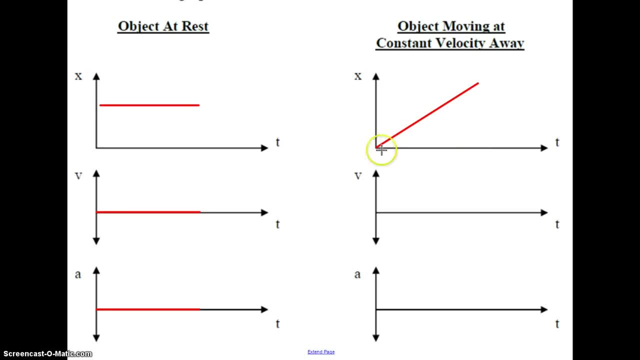 That's the only direction time can move. Okay, And the fact that the line is straight means that the rate of change of the displacement or distance is staying constant, And of course that means constant velocity. If that's true, then on our VT graph we're going to have some non-zero velocity over that same time interval. 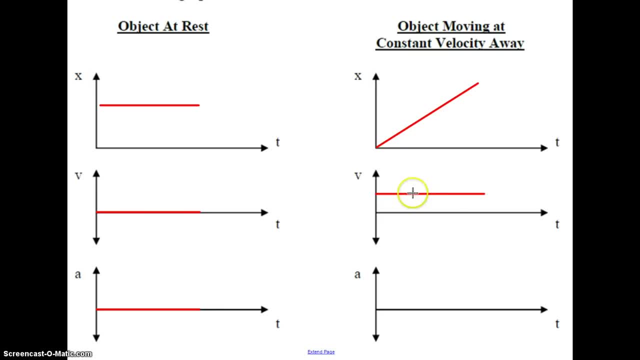 And it should be obvious to us that that velocity remains constant. You notice here that this horizontal line is about the same time interval And it should be obvious to us that that velocity remains constant. This horizontal line is above the time axis. The slope of this line is positive. up here on the XT graph. 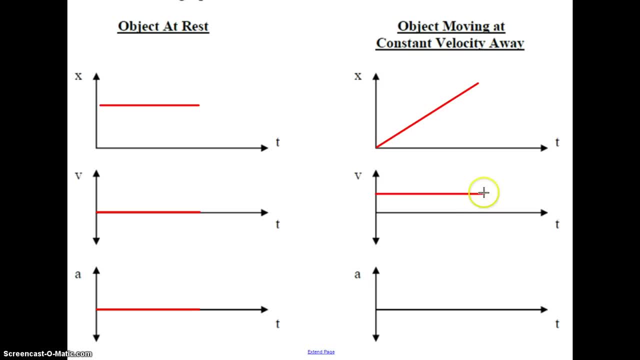 So our velocity is positive on our VT graph. We still are not accelerating. This object is not speeding up or slowing down, So its acceleration value is zero. So this would be a horizontal line on the time axis. Moving on to our next scenario, 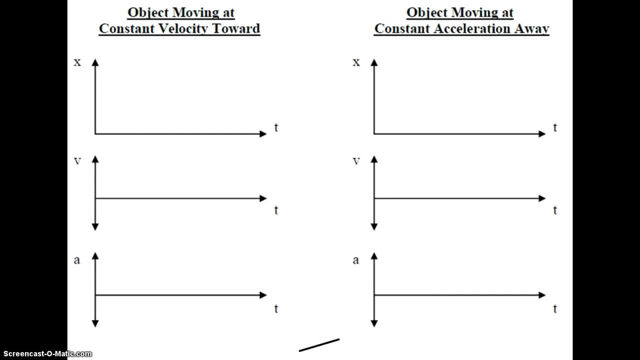 Moving on to our next scenario. Moving on to our next scenario: Object moving at constant velocity toward Object moving at constant velocity toward. Well, constant velocity means our line is going to be straight. Well, constant velocity means our line is going to be straight. 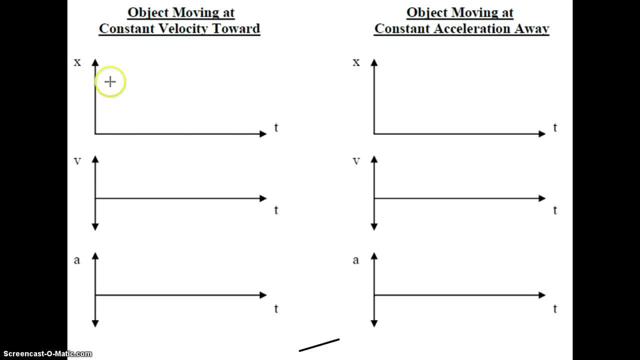 Toward means that our X numbers, our distance numbers, are going to be decreasing. Toward means that our X numbers, our distance numbers, are going to be decreasing. Toward means that our X numbers, our distance numbers, are going to be decreasing. 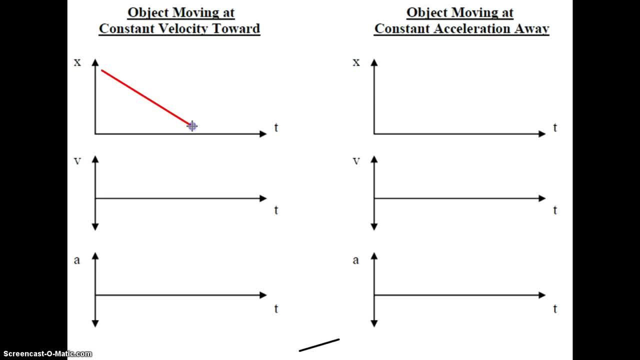 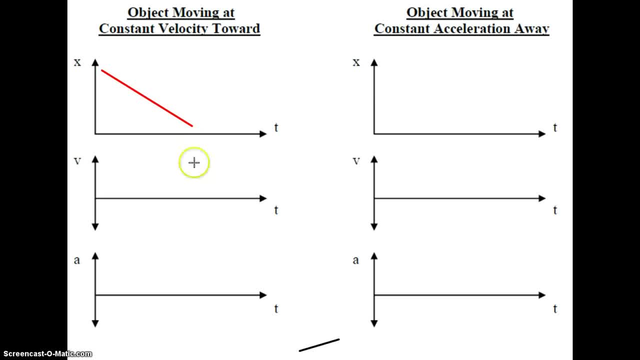 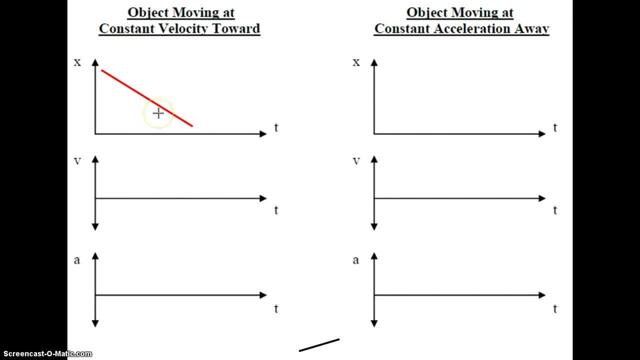 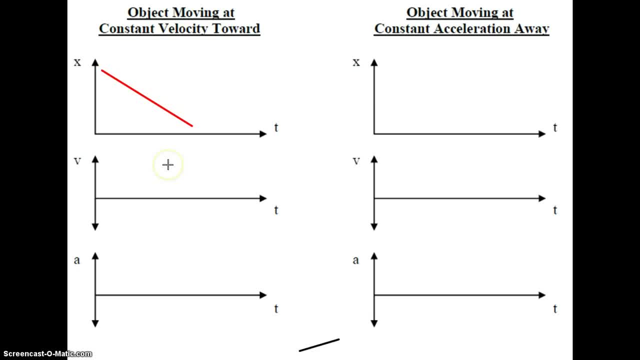 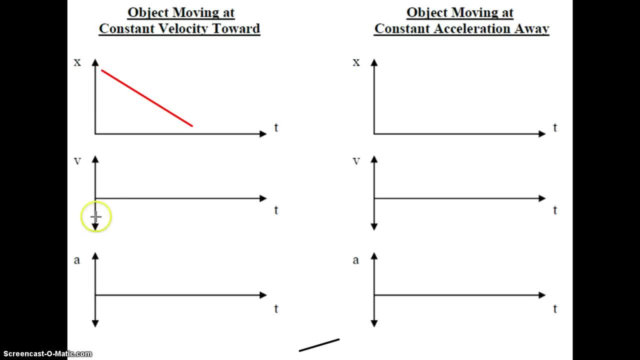 Well, constant velocity again means that we're going to have a horizontal straight line. Well, constant velocity again means that we're going to have a horizontal straight line. This time, though, our horizontal straight line is below the time axis. This time, though, our horizontal straight line is below the time axis. 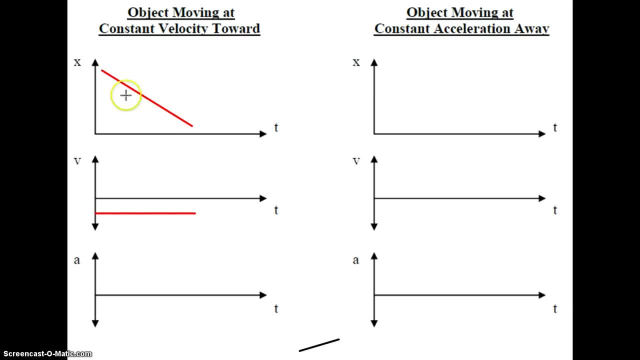 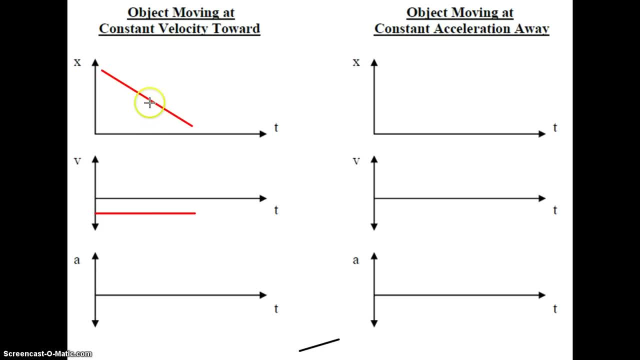 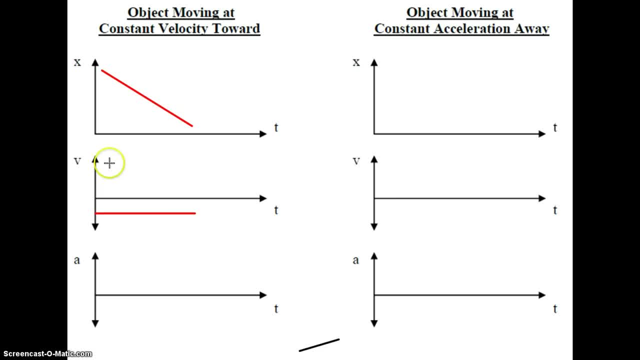 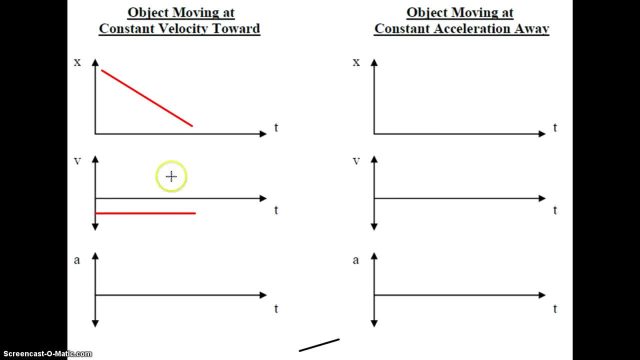 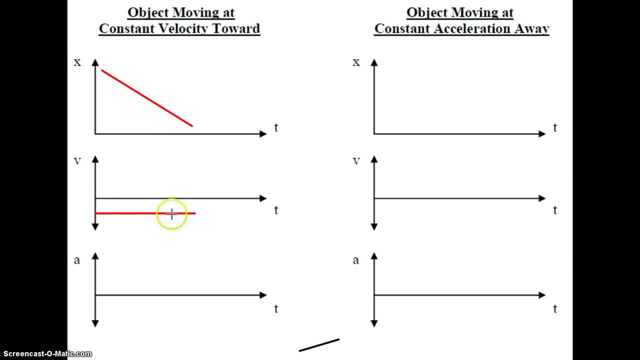 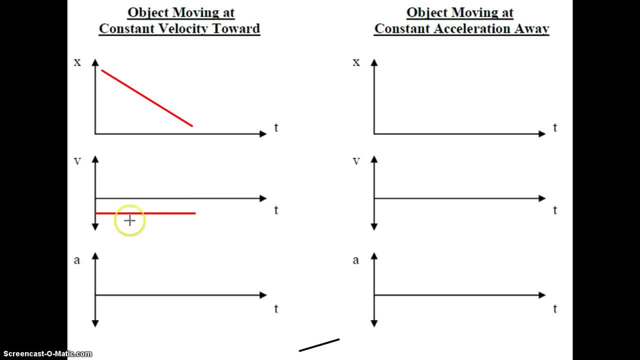 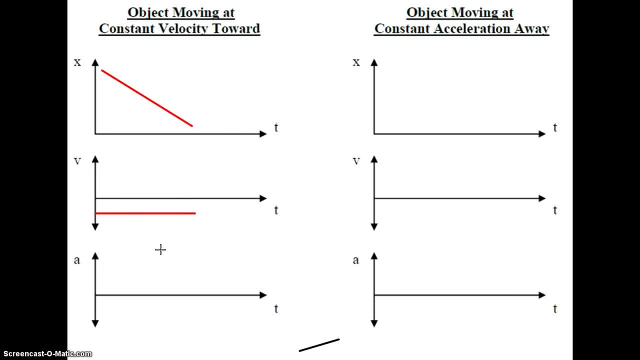 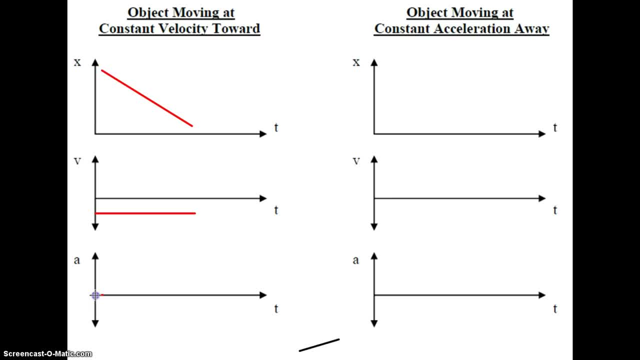 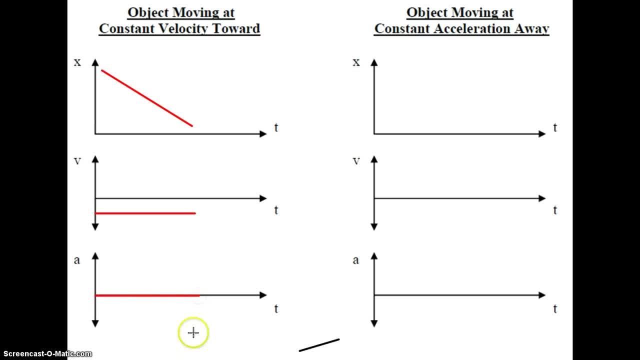 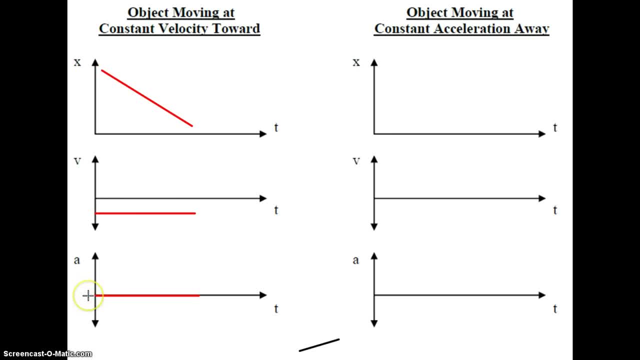 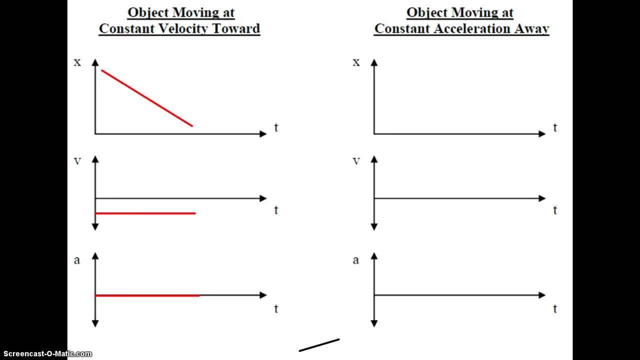 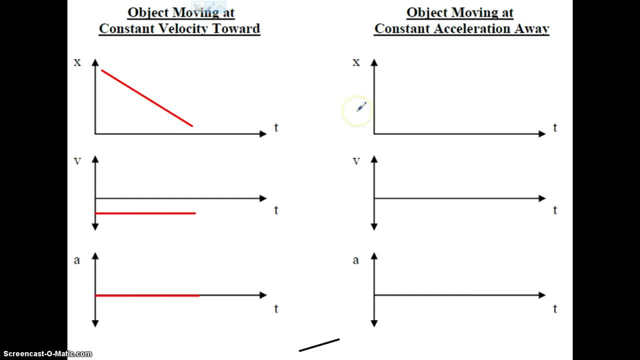 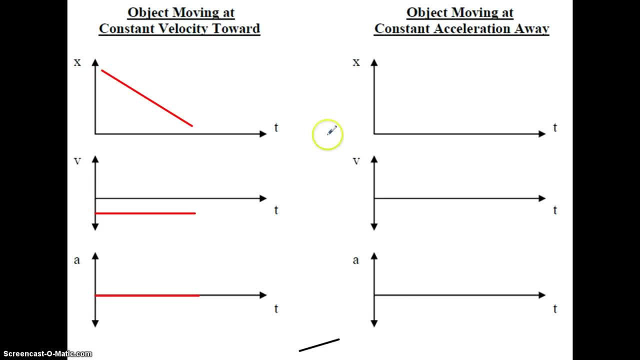 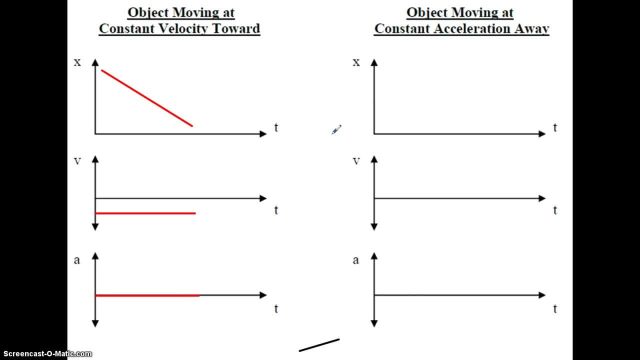 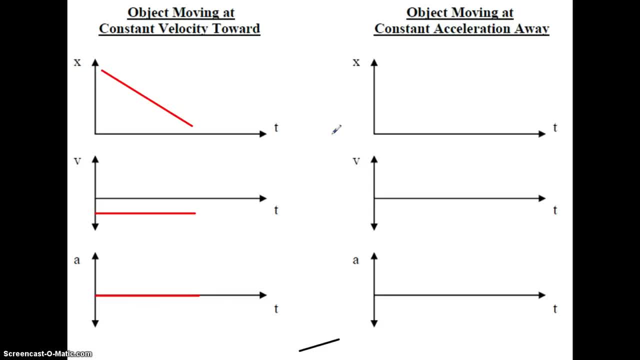 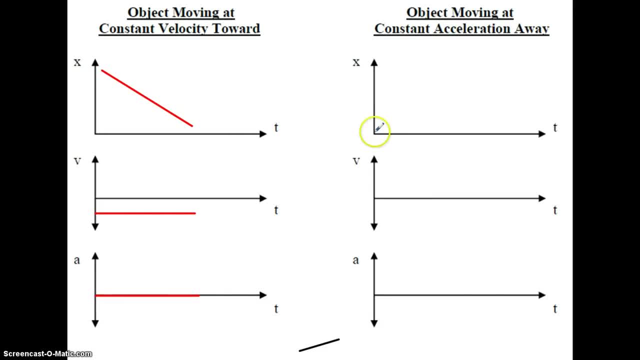 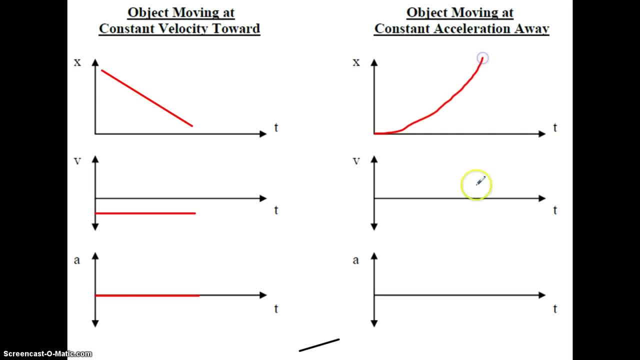 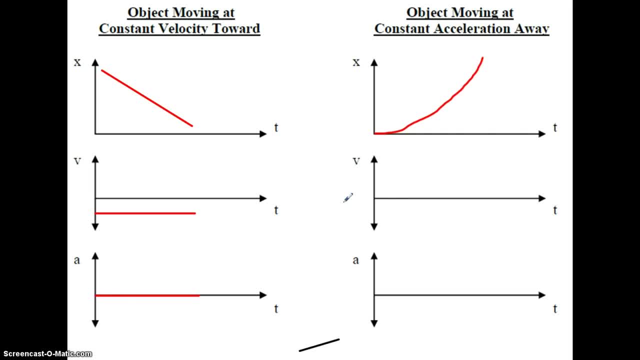 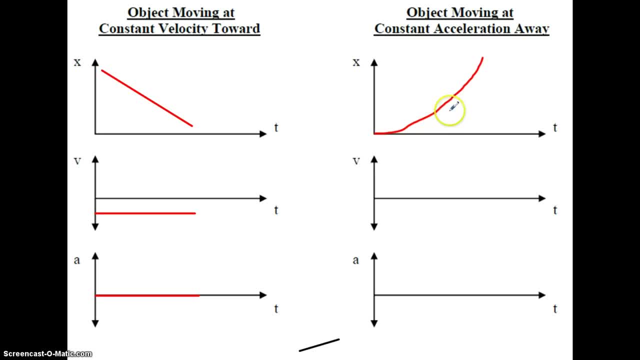 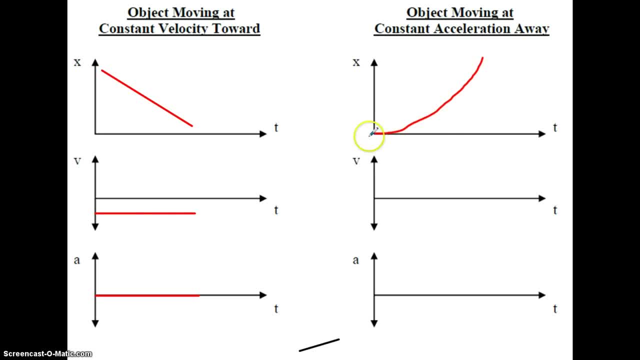 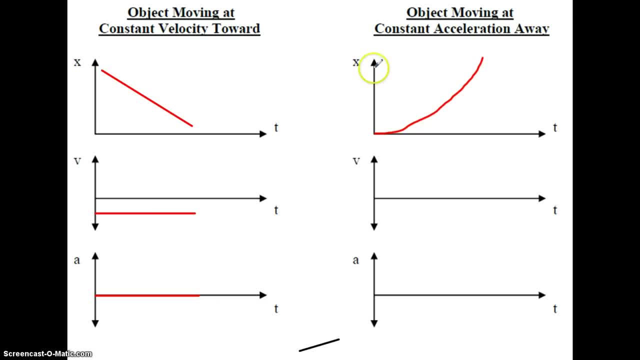 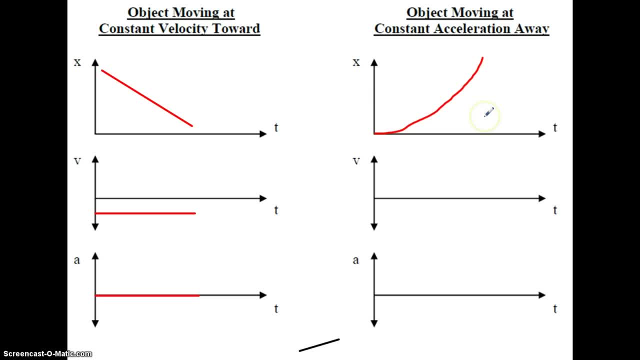 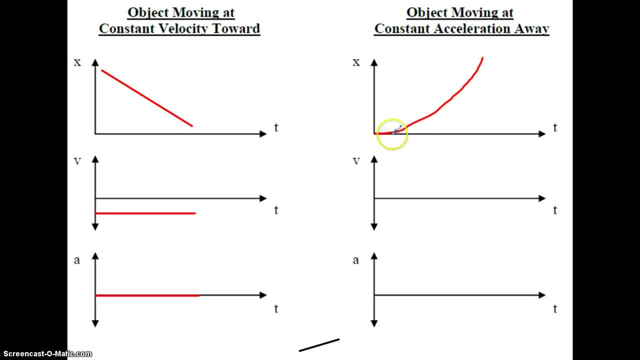 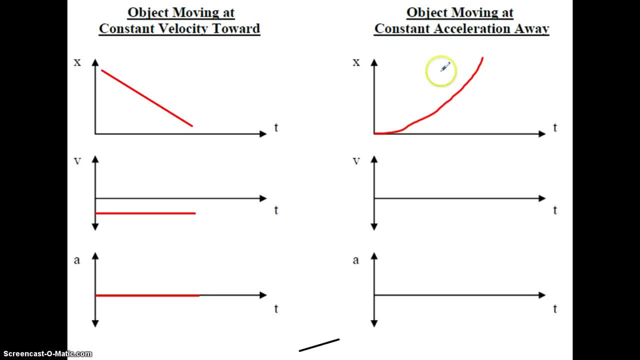 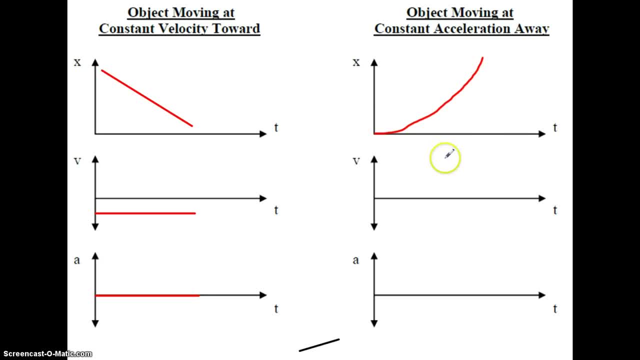 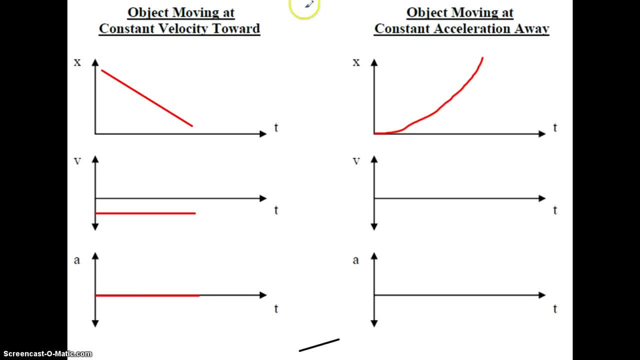 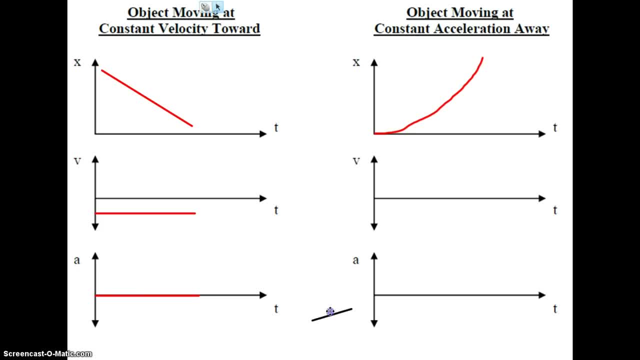 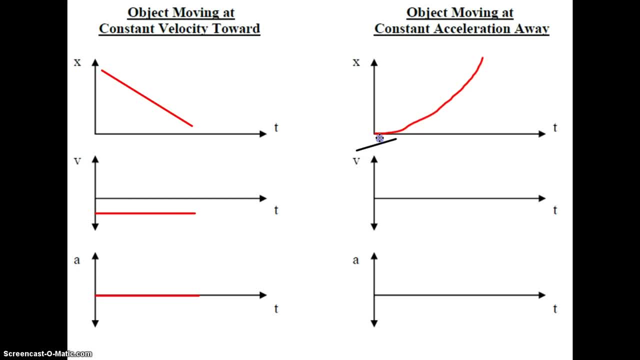 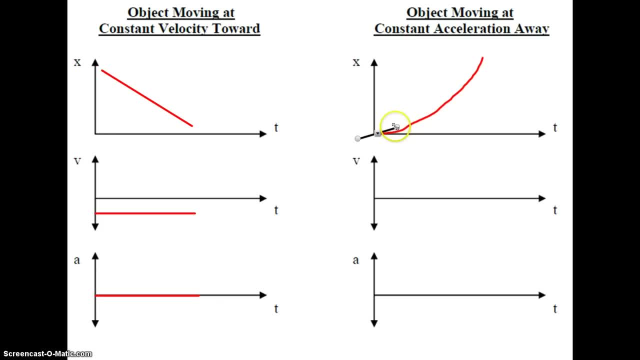 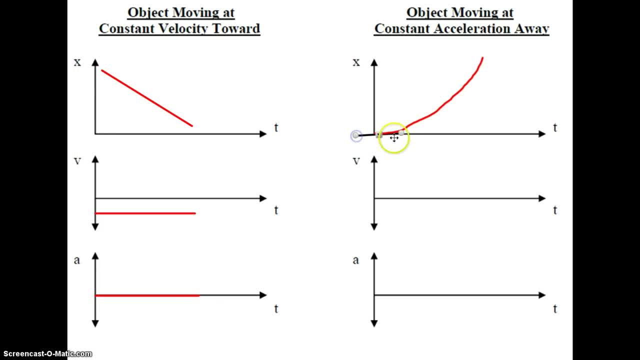 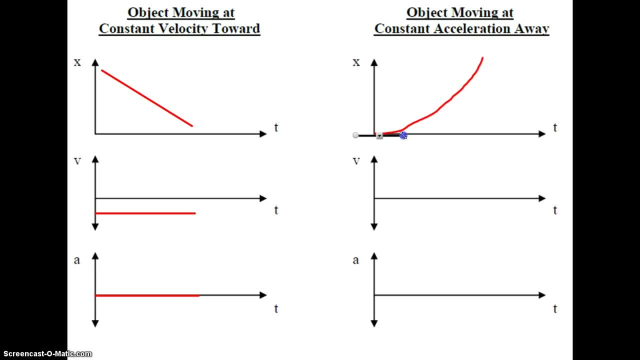 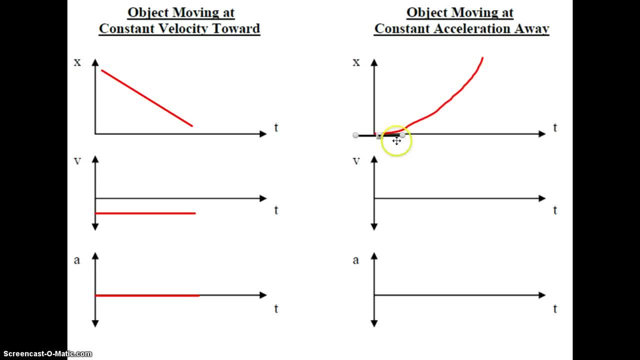 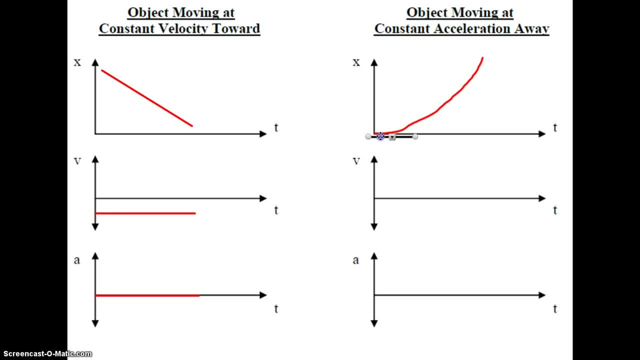 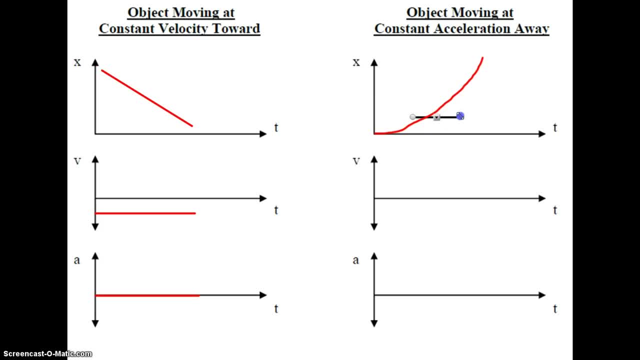 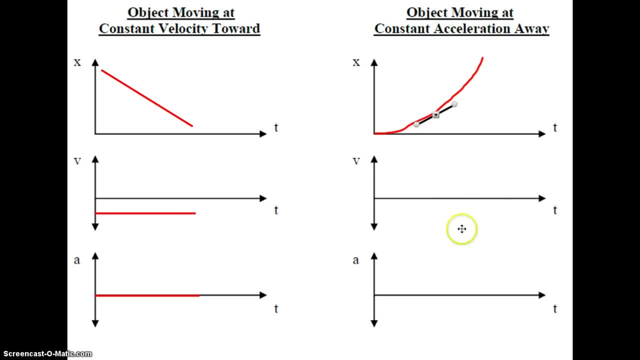 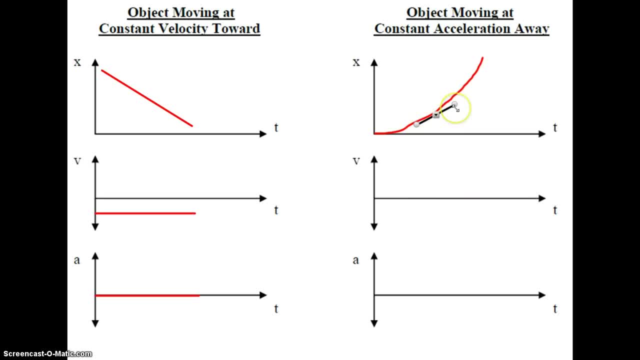 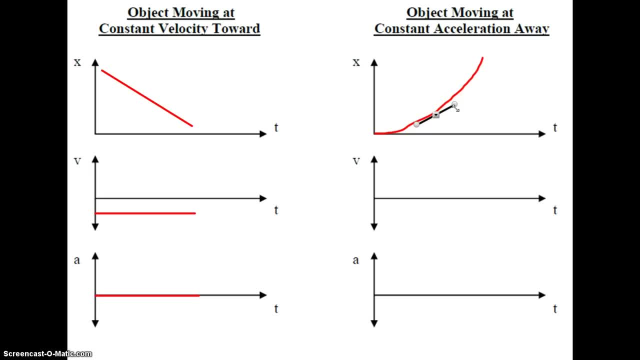 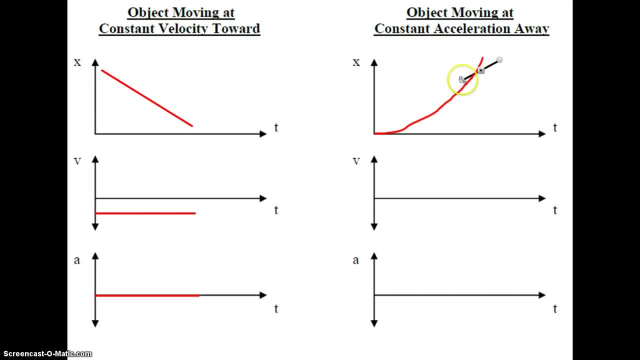 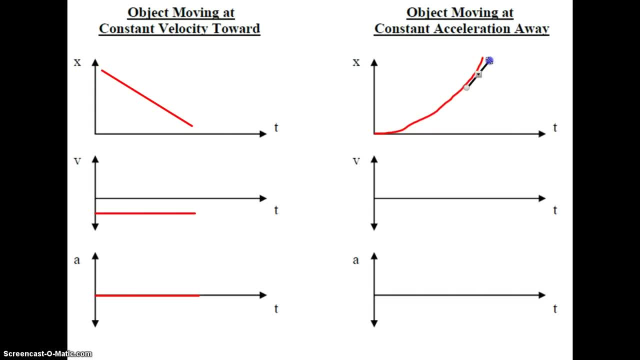 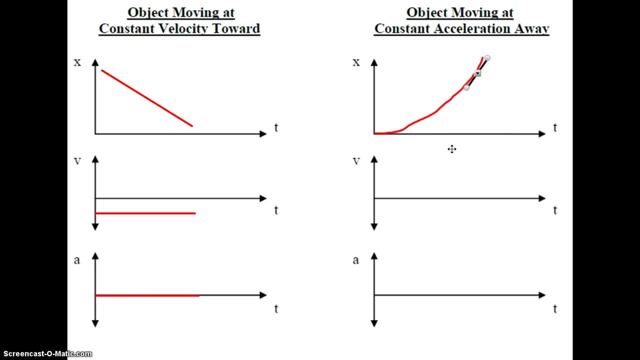 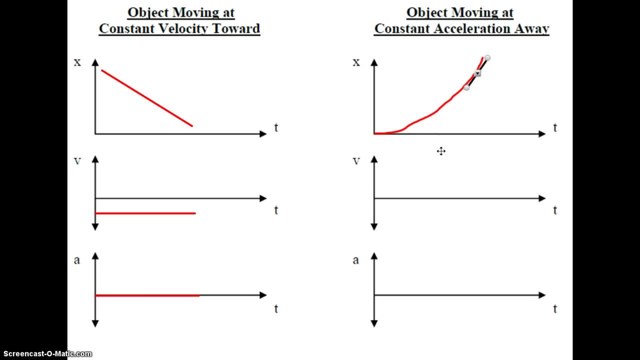 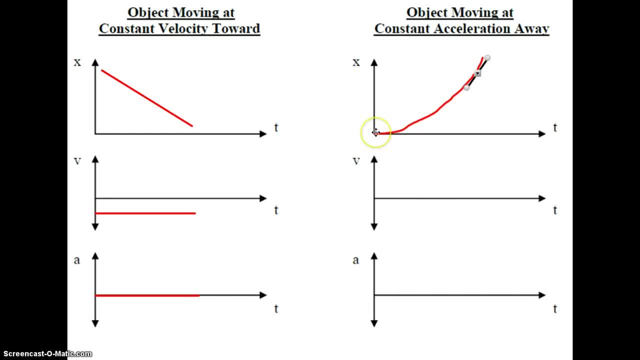 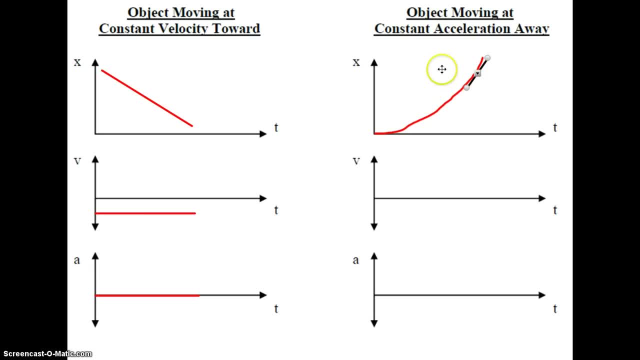 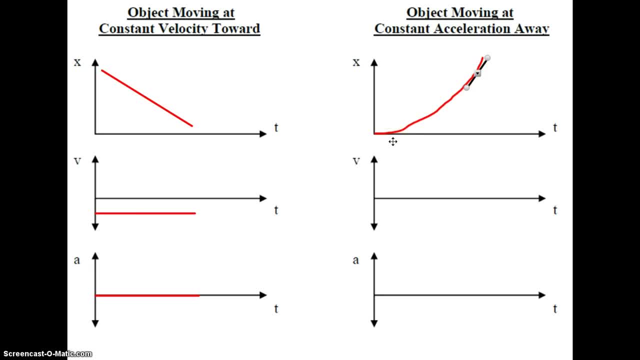 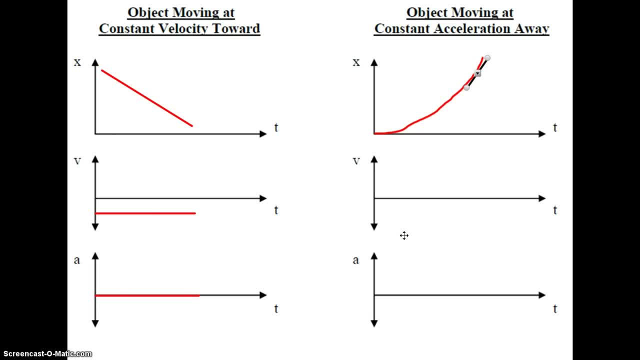 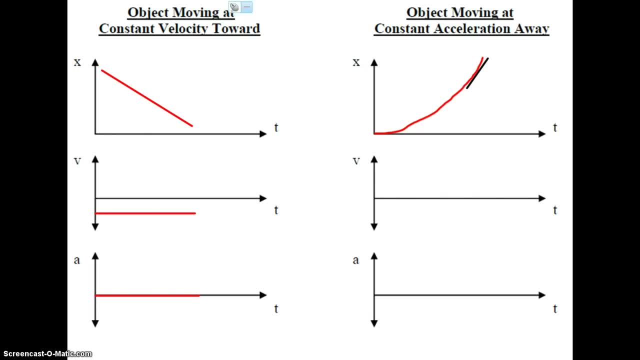 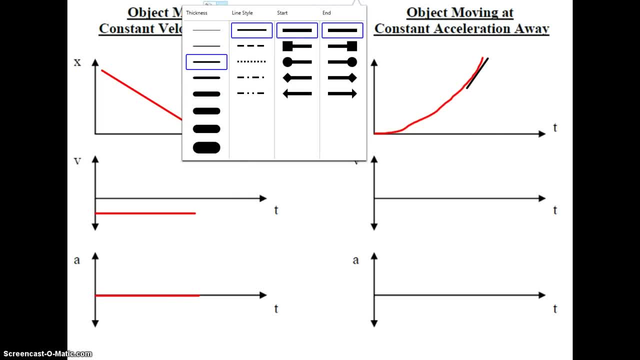 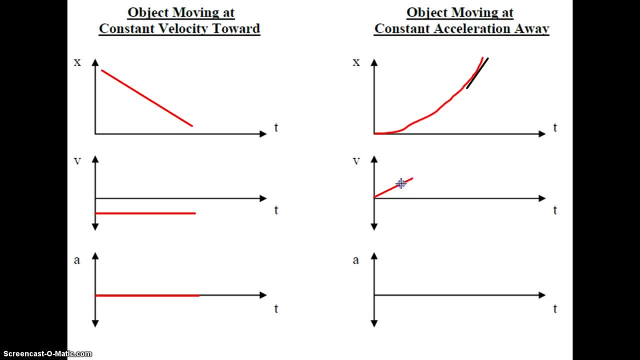 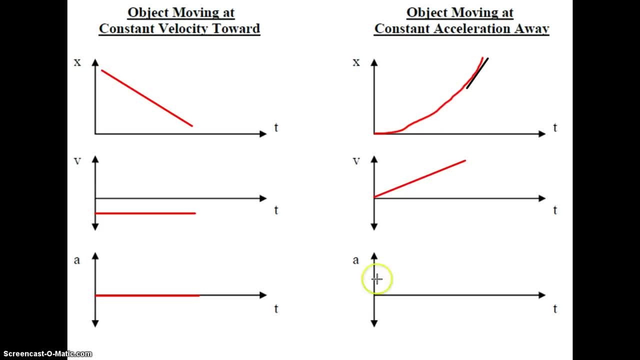 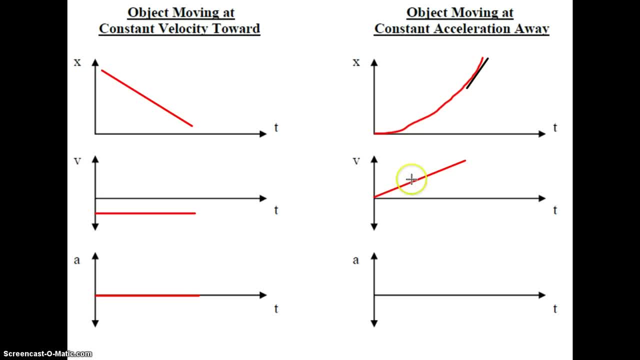 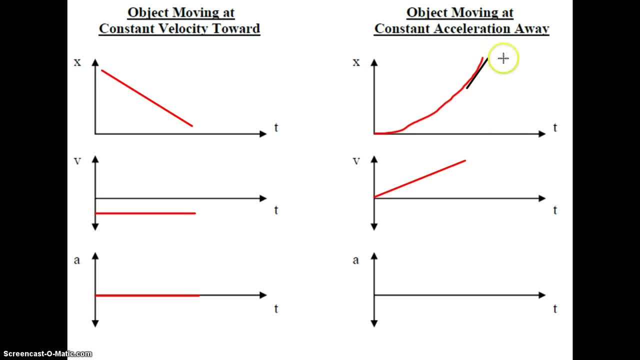 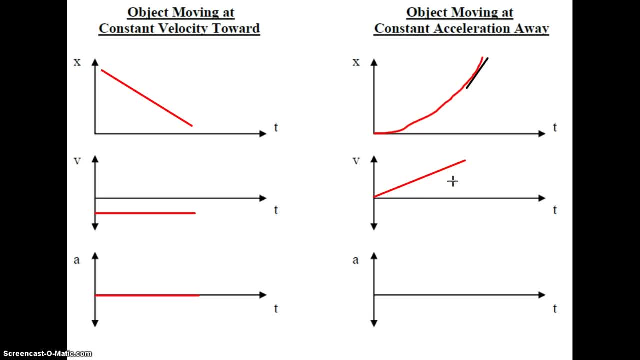 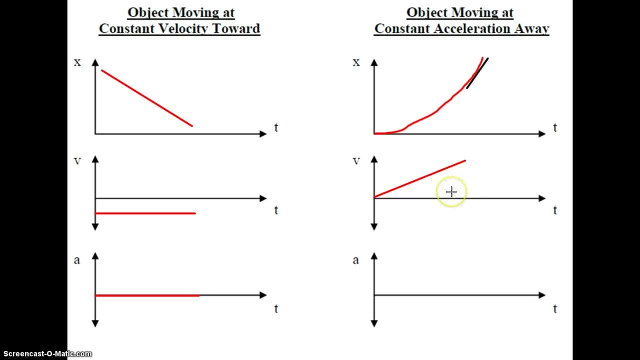 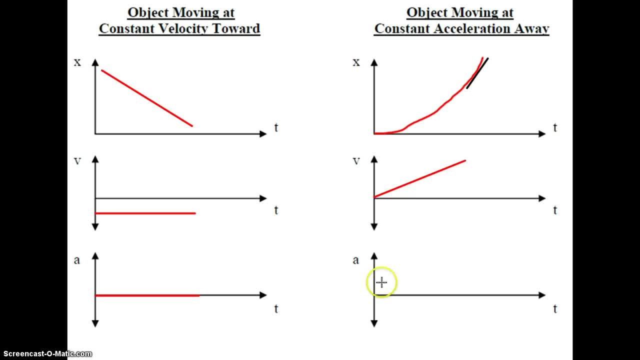 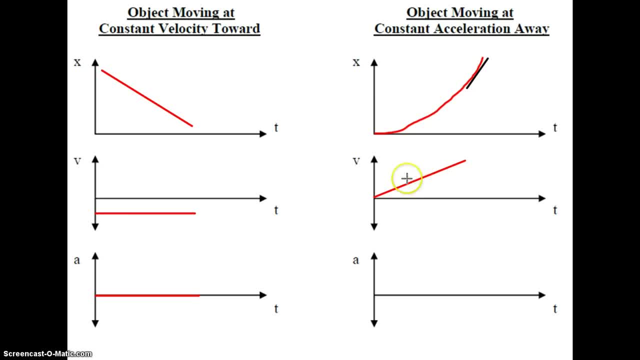 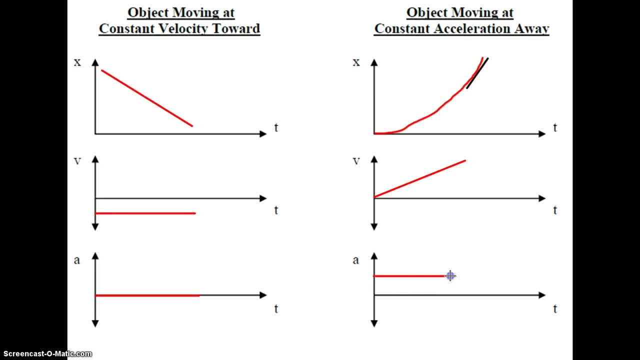 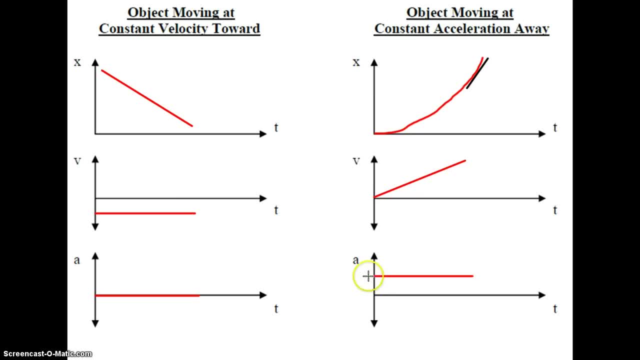 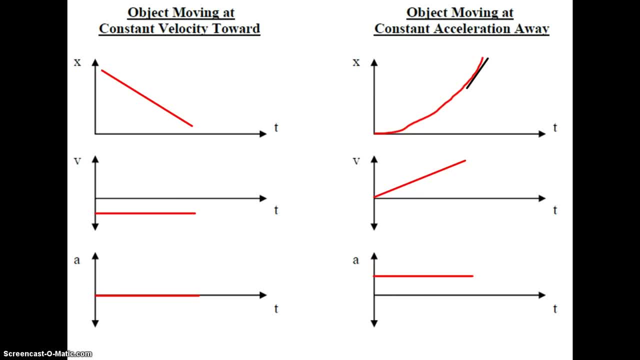 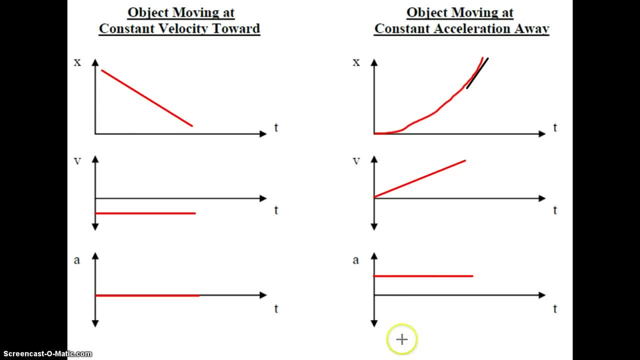 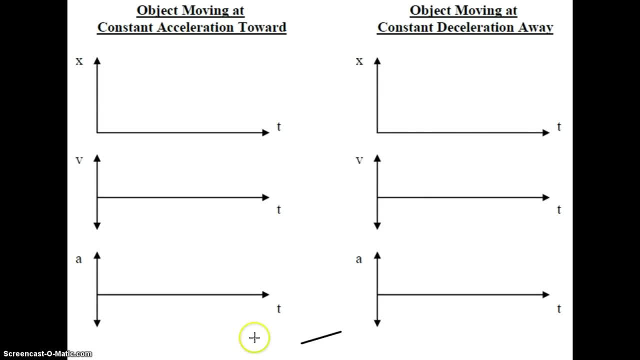 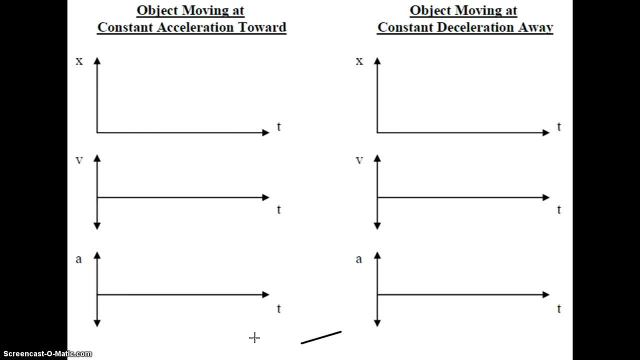 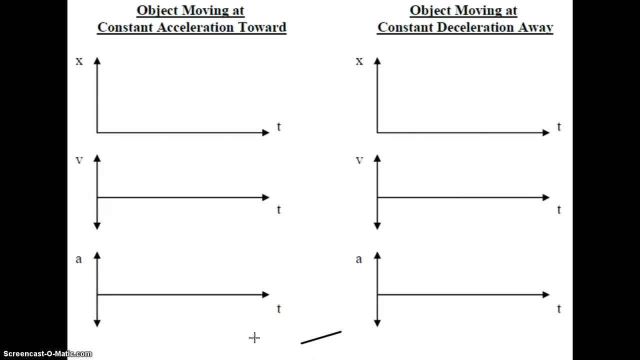 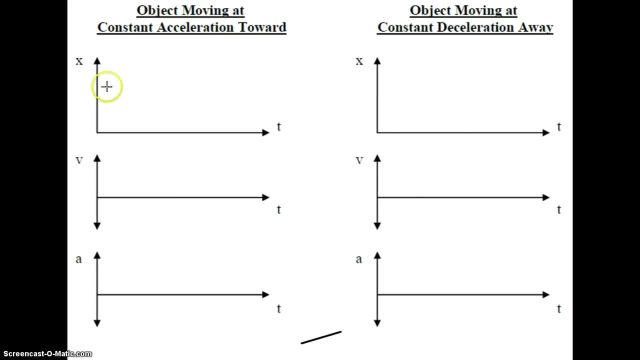 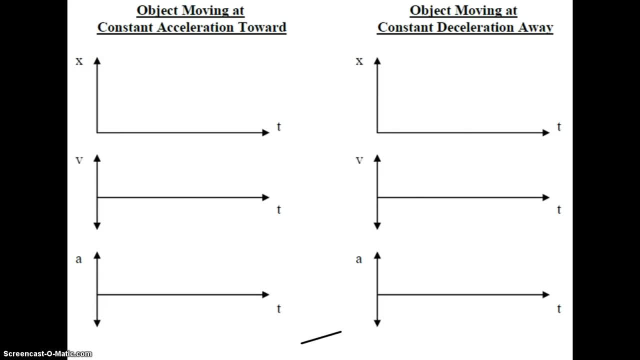 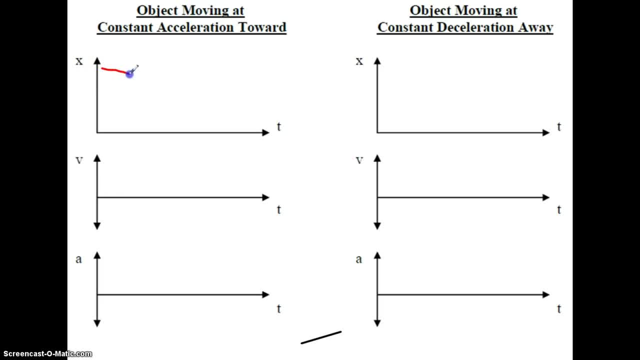 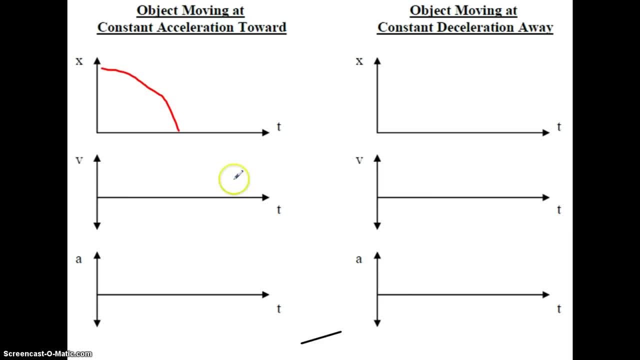 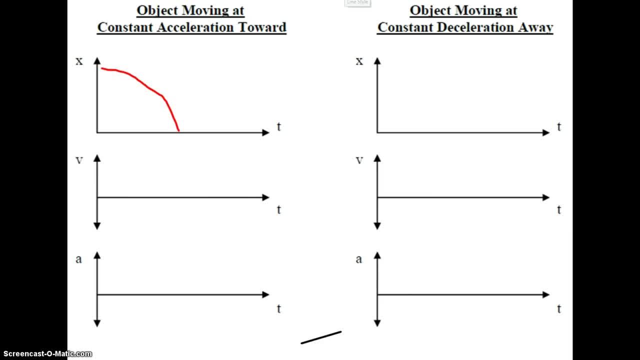 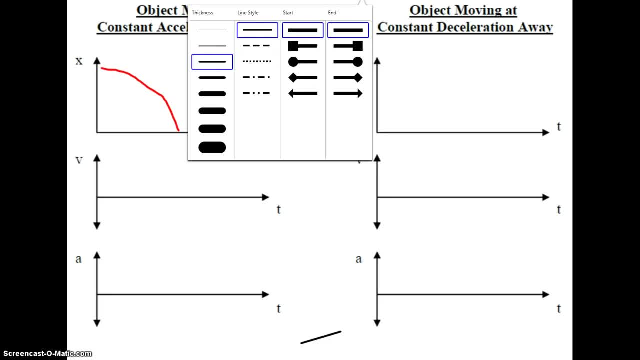 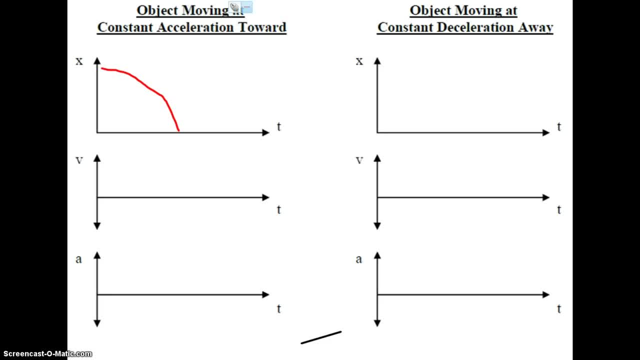 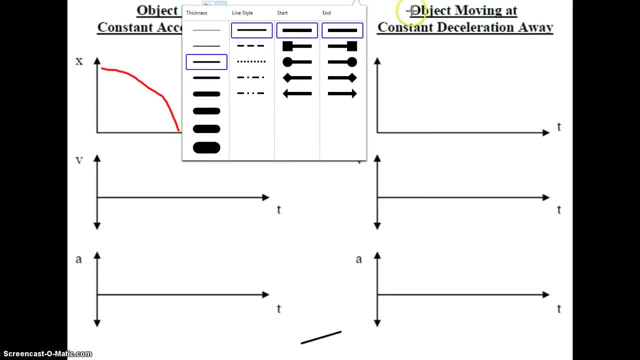 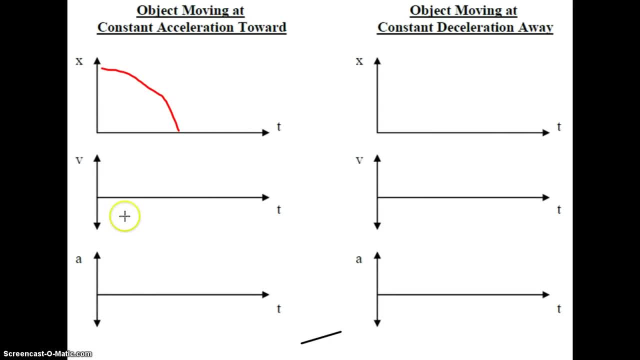 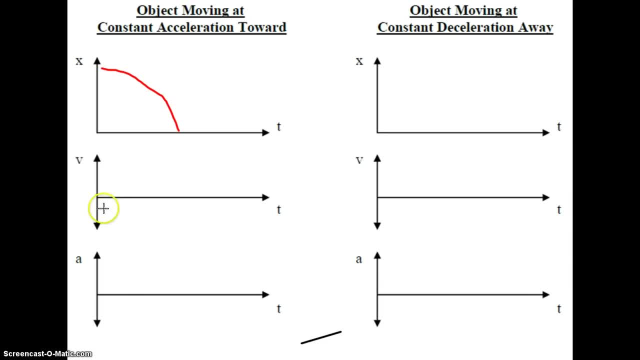 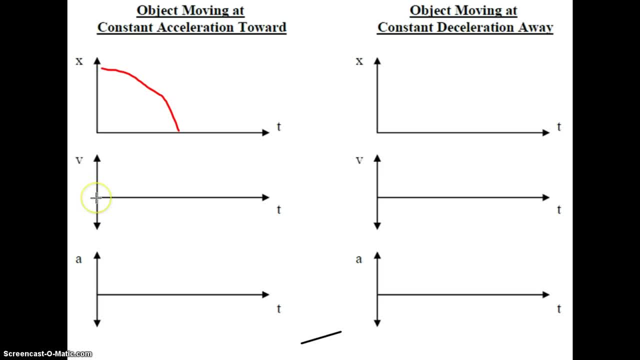 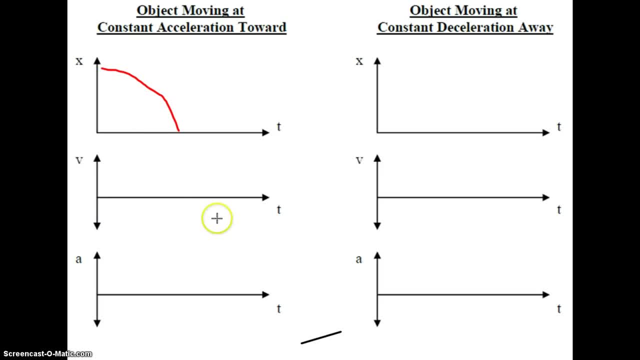 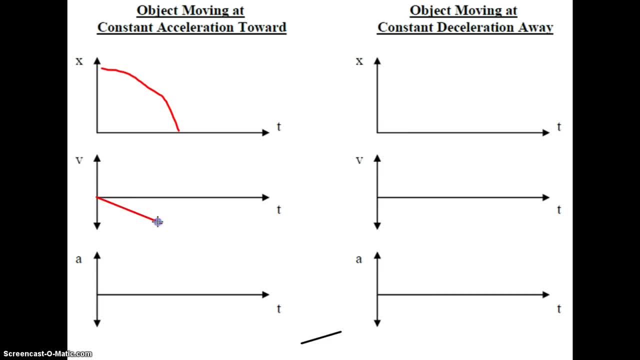 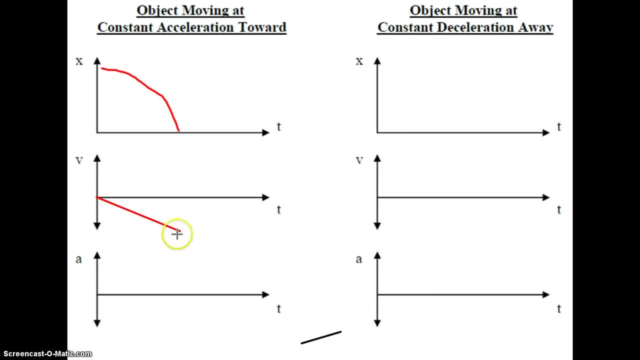 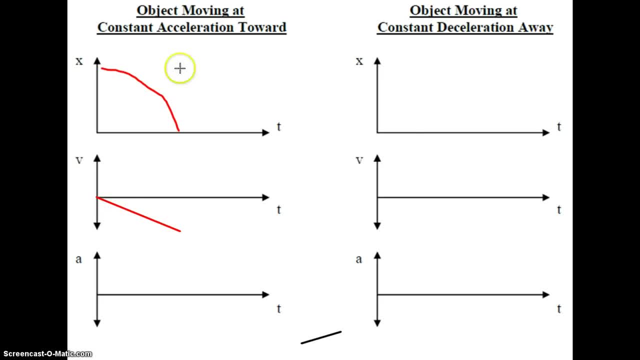 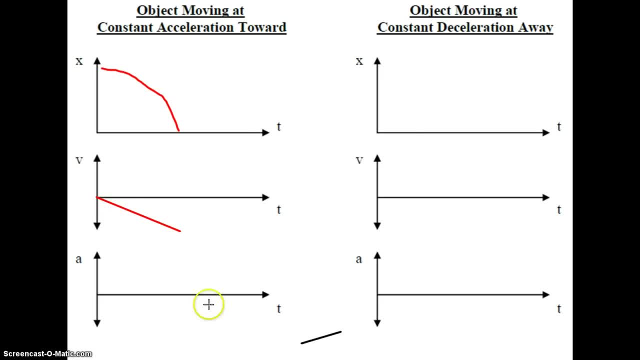 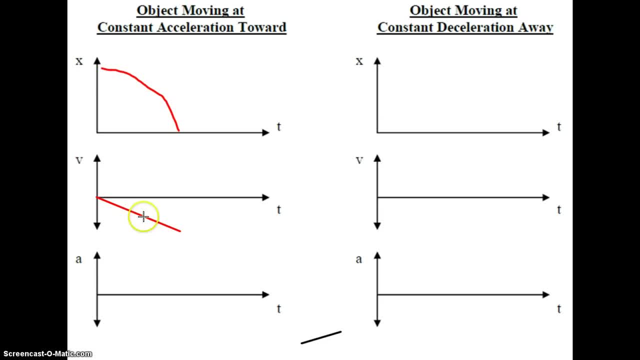 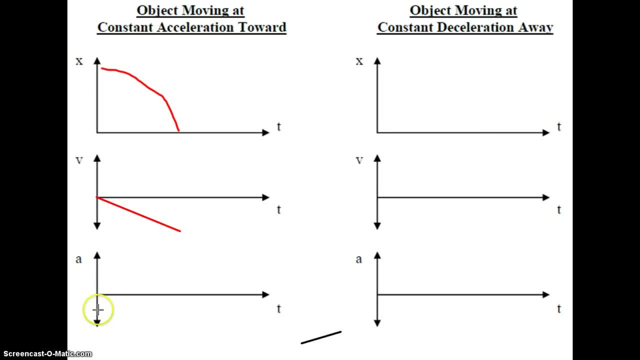 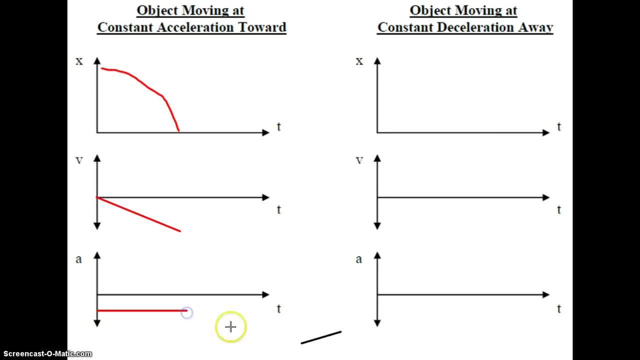 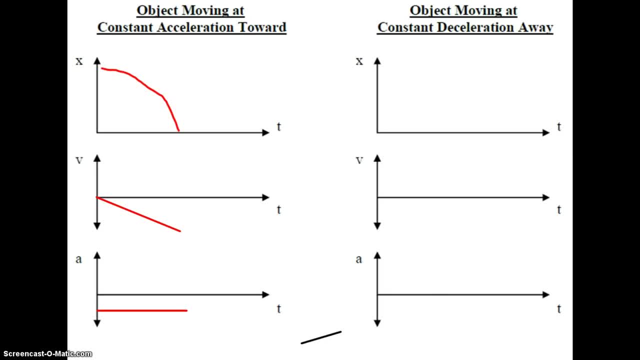 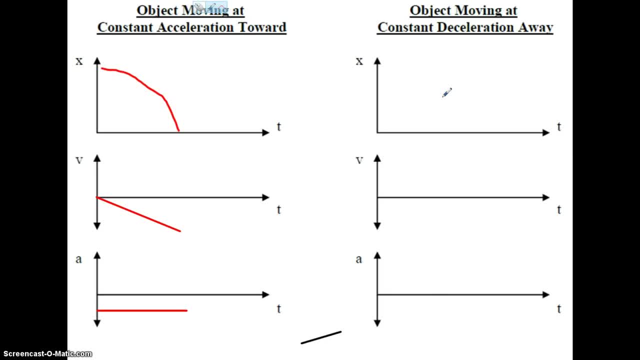 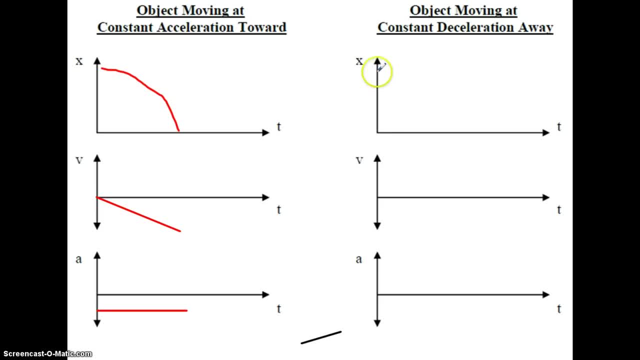 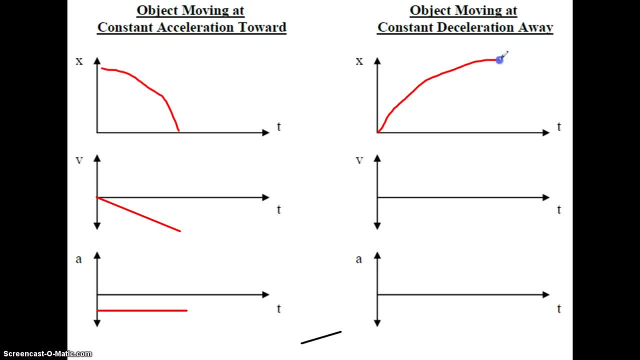 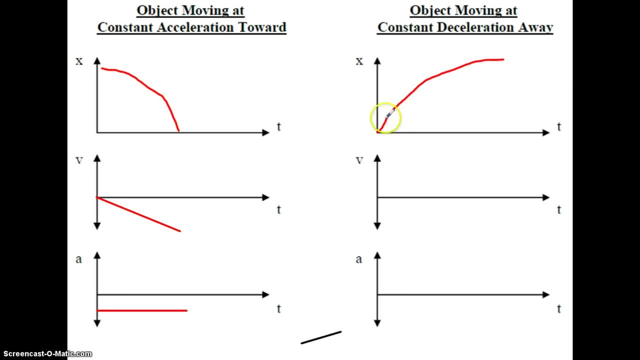 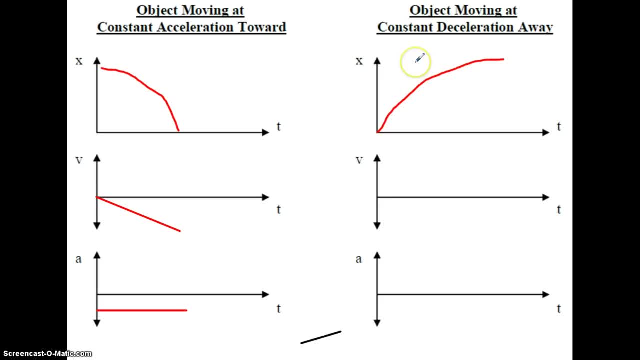 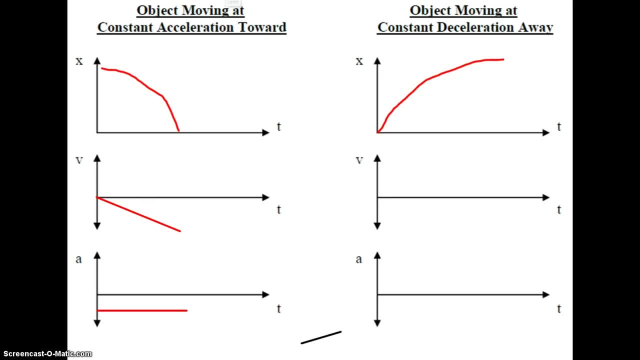 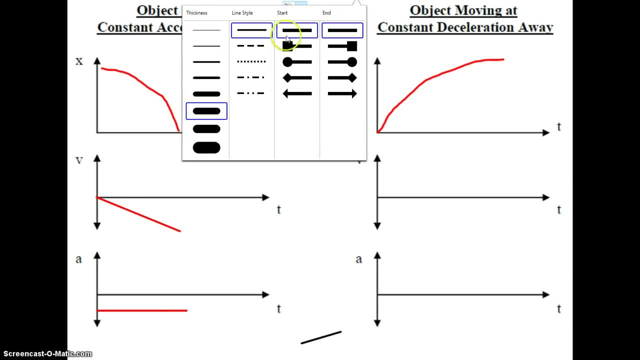 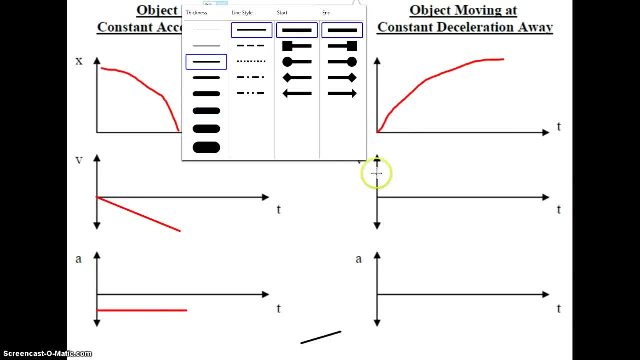 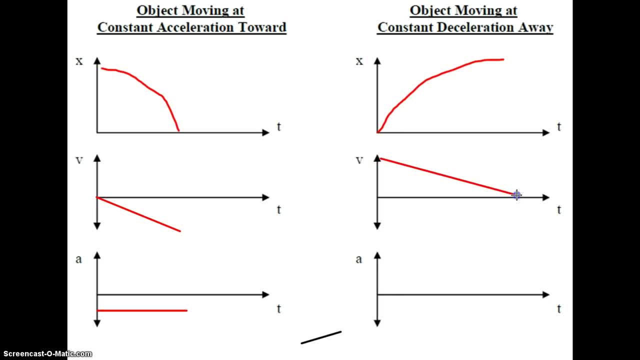 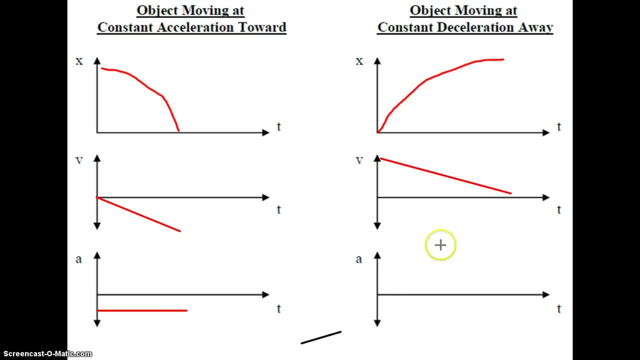 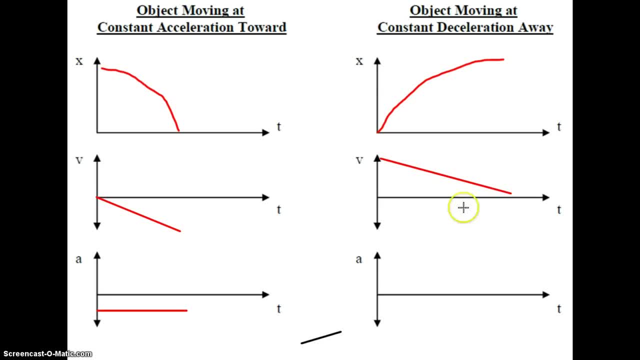 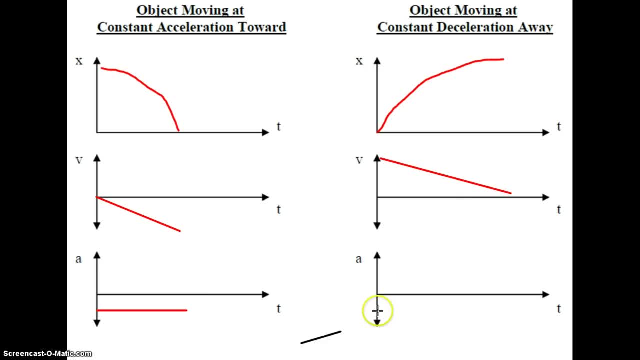 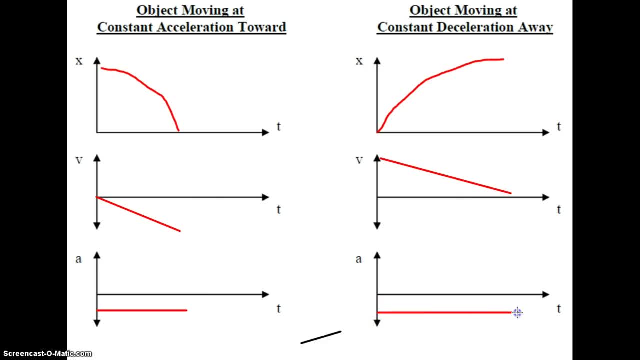 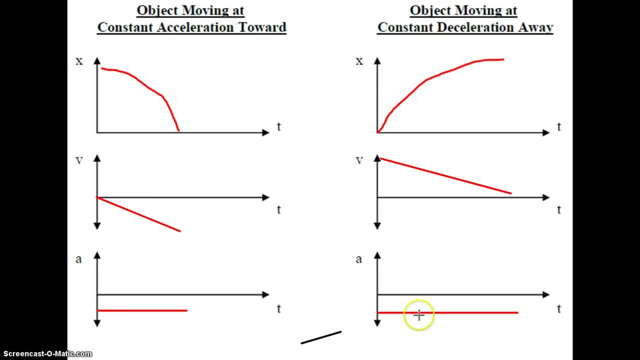 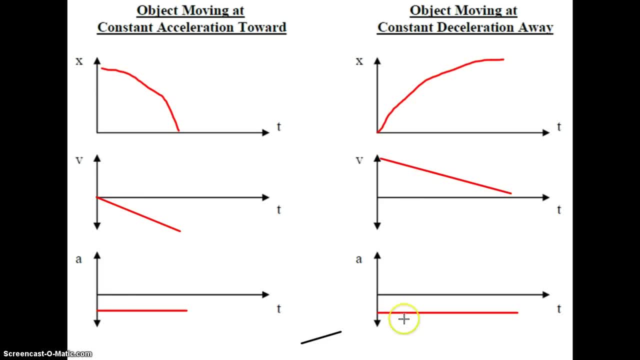 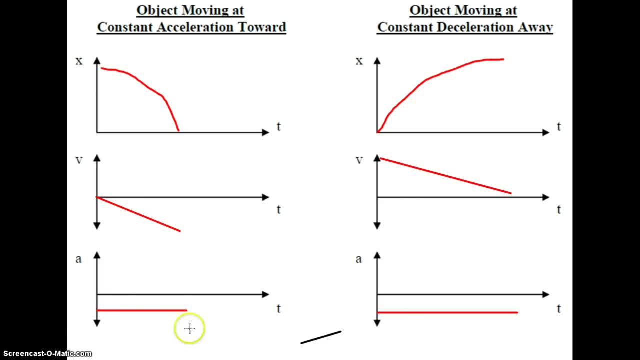 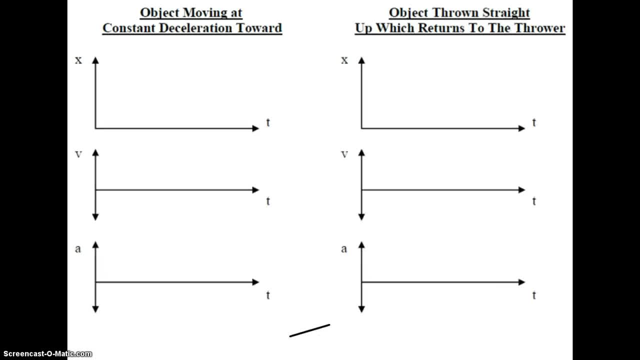 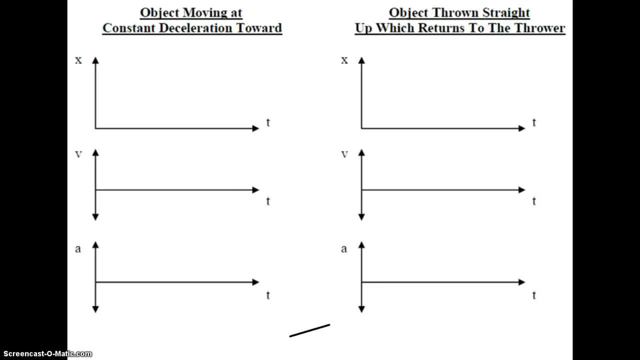 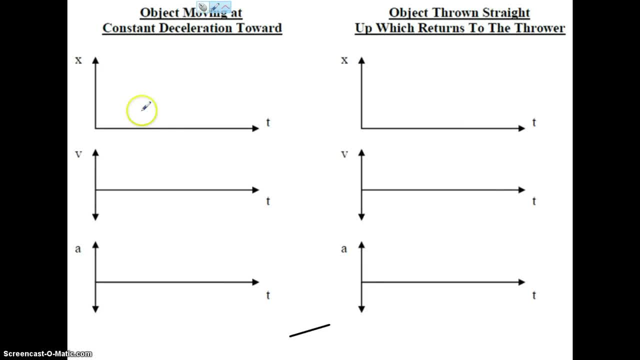 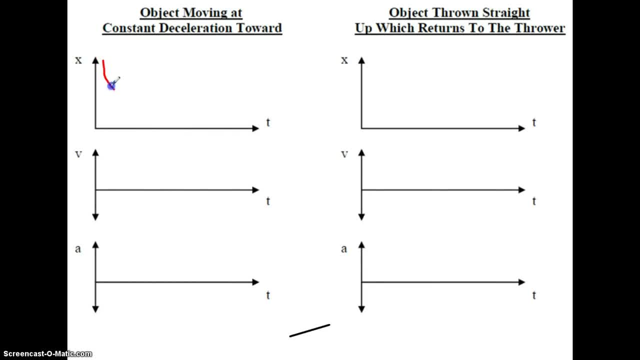 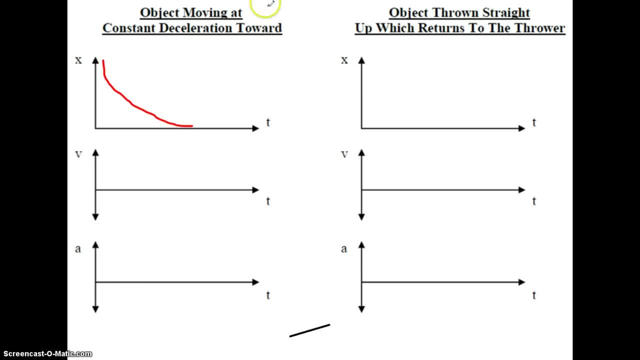